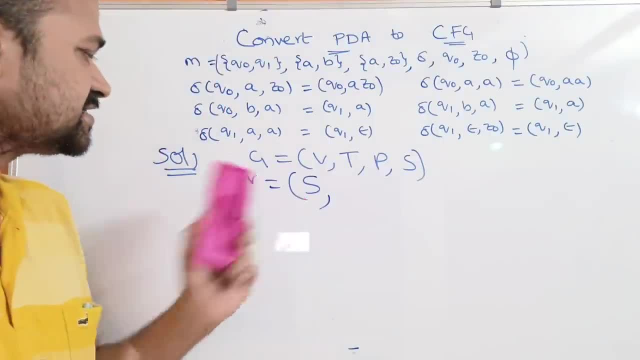 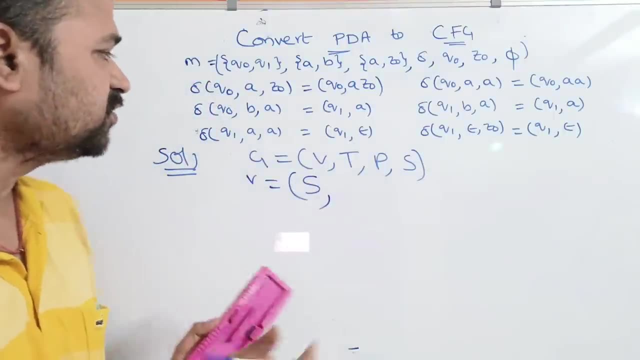 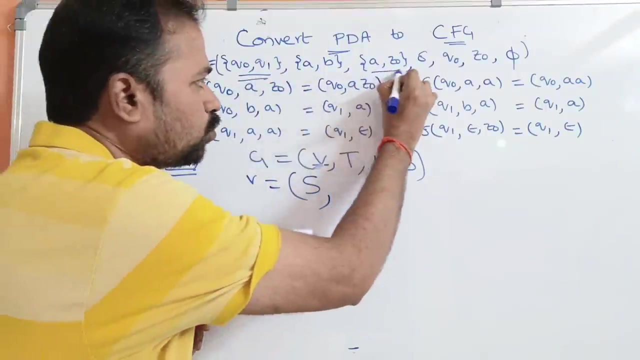 represented with the help of some capital N's likewise, So v is equal to s comma. Next we have to write the remaining variables here. So for writing the variables, what we have to do is we have to combine. we have to combine this q with tau. 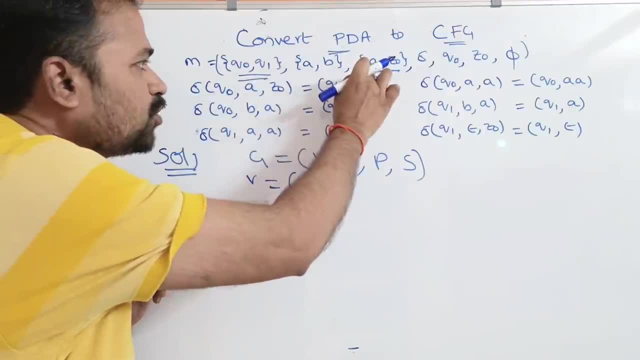 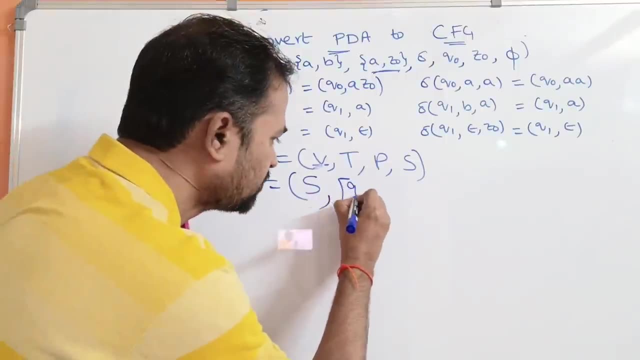 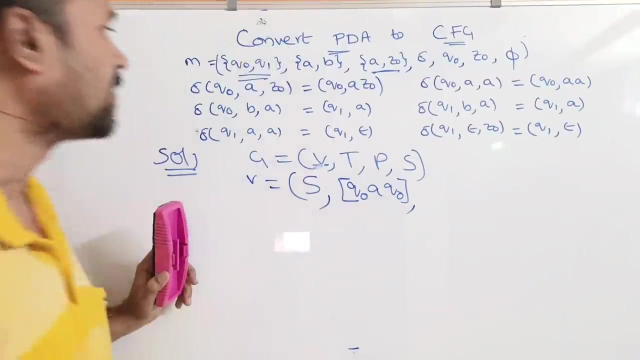 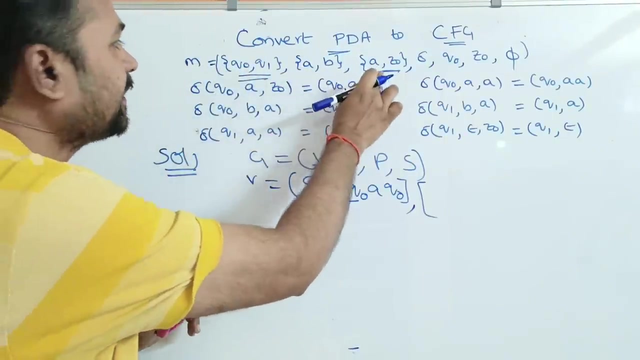 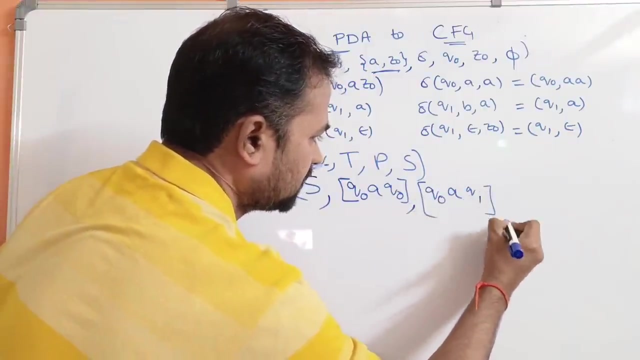 with down. so here the first combination is: q naught a q naught a q naught. so within the square bracket side. so q naught a q naught. so this is one more variable. so next one: q naught. q naught a q1. so q naught a q1. so next one. so starting with q naught is: 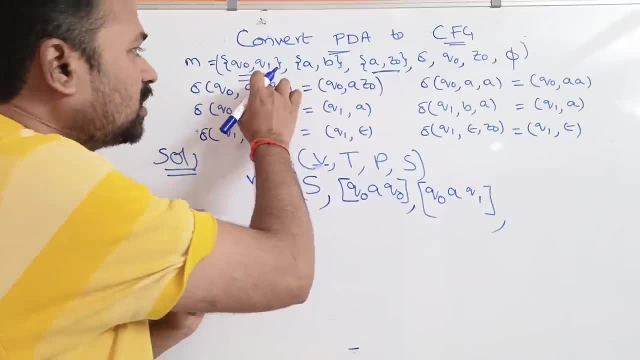 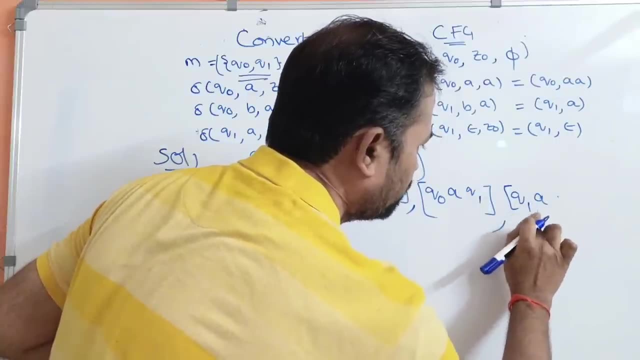 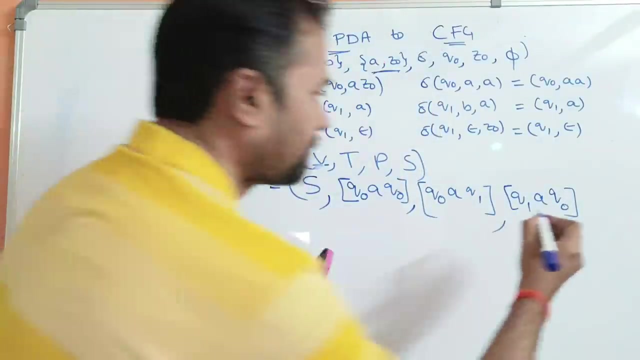 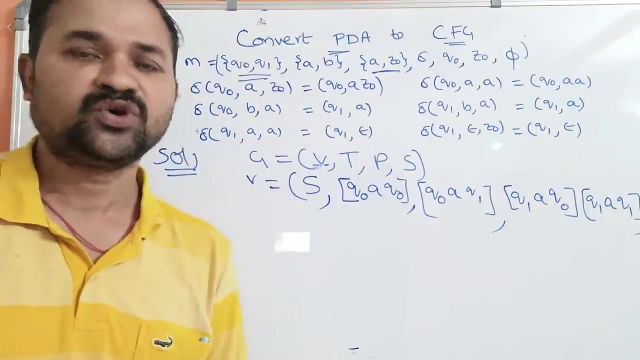 now let us start with q1. so combine q1 with a, so q1 a q naught, so q1 a q naught. so next one: q1 a q1, so q1 a q1. so next we have to take z naught as the middle symbol. 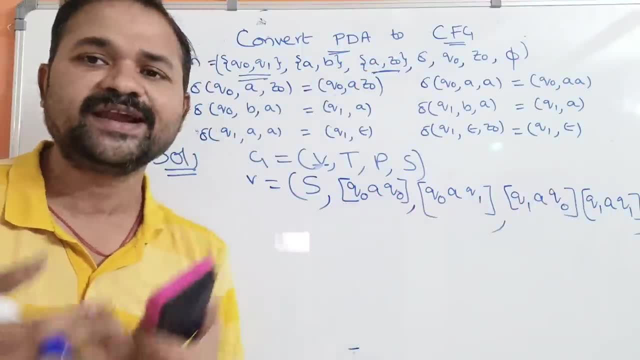 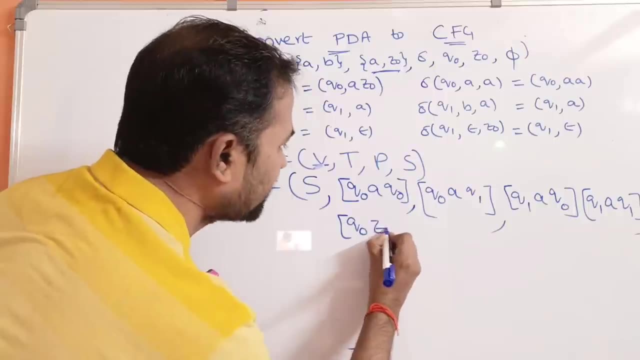 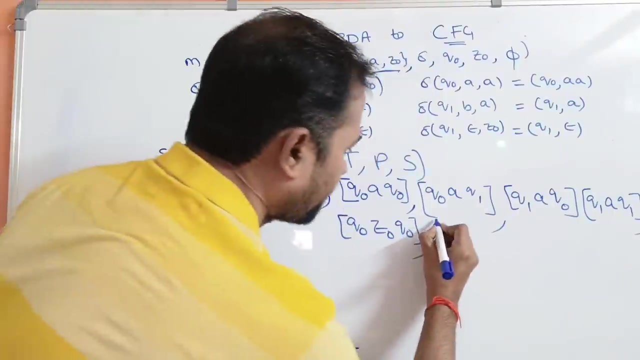 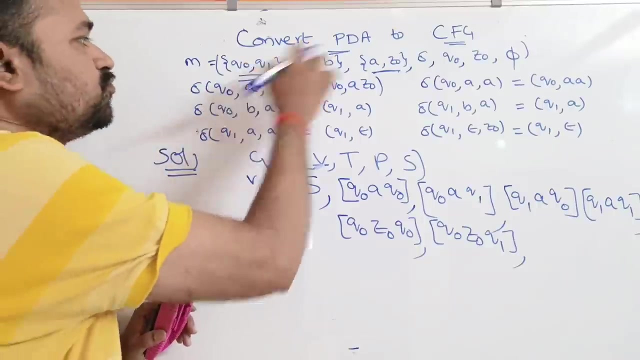 so till now we have taken a as the middle symbol. next we have to take this z naught as the middle symbol. so q naught z naught, q naught, comma. next q naught z naught, q1. q naught z naught, q1, next one: q1 z naught, q naught, so q1 z naught. 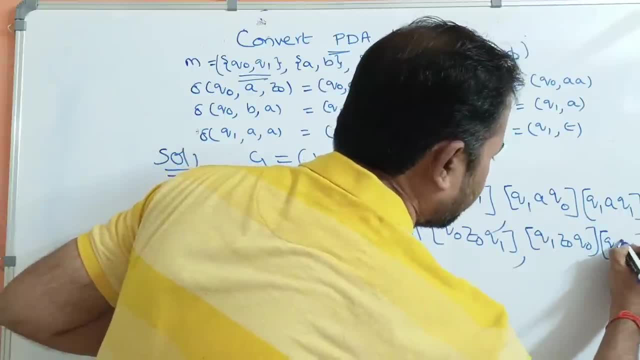 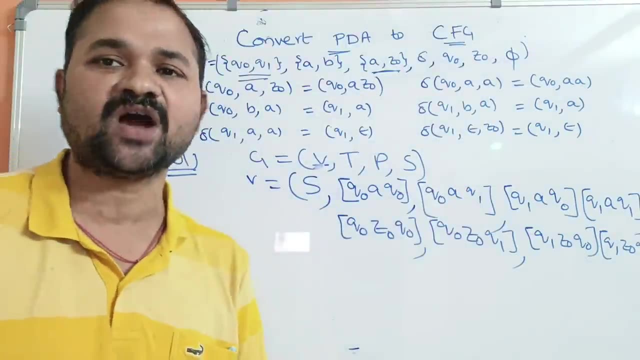 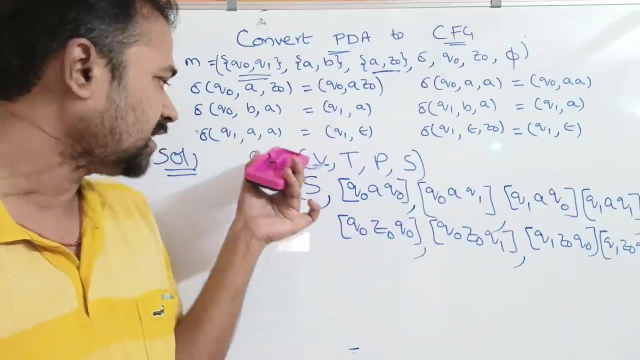 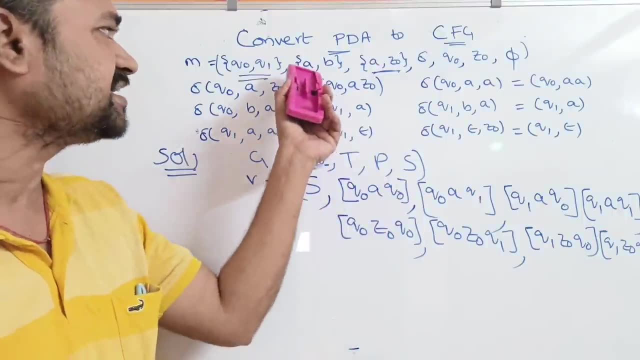 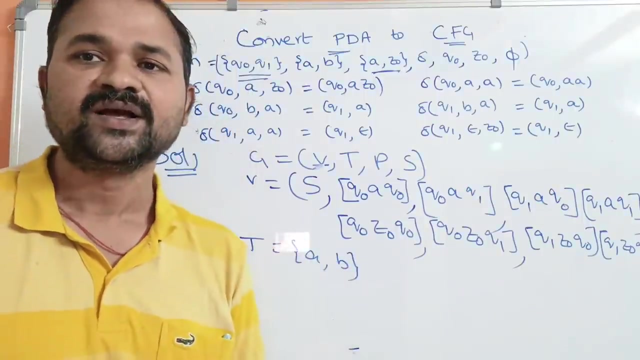 13 Kites for what we have pointed out, for these are part of the integral 식b. Next we have to write the terminal symbols. so there is no difference in the terminal symbols. so here also the terminal symbols are a and b, only a and b only. next predictions. 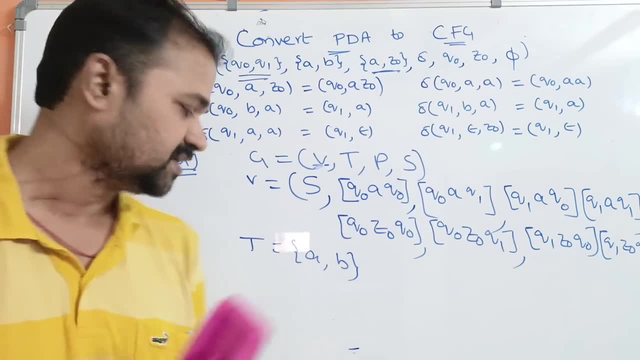 let us write predictions later, after writing the start symbol. so let us write the start symbol now. let us start symbol. s implies that means start before we write the first detta and after this element we need to write the initial value. So let us write the initial state. beyond this, 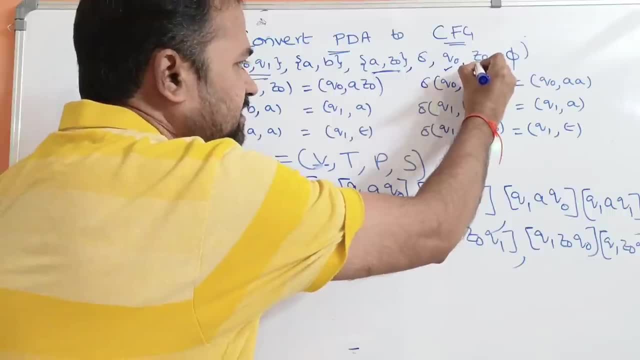 the initial state of this thing because capital S is different than the initial suffix order, space f and s port per sample right and if we return to the initial state which we have here, is is q naught and the stack initially contains z naught, So we can write it as q naught. 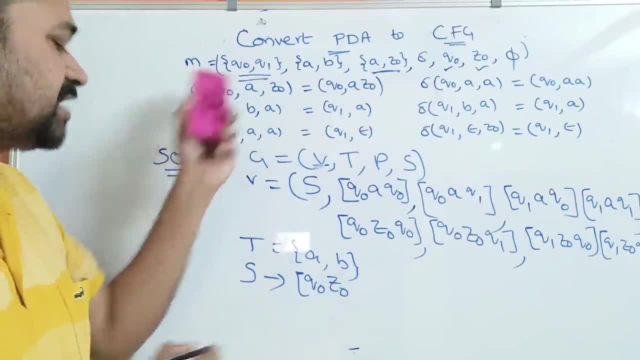 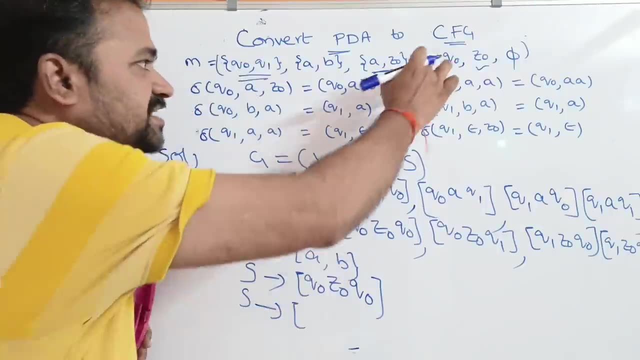 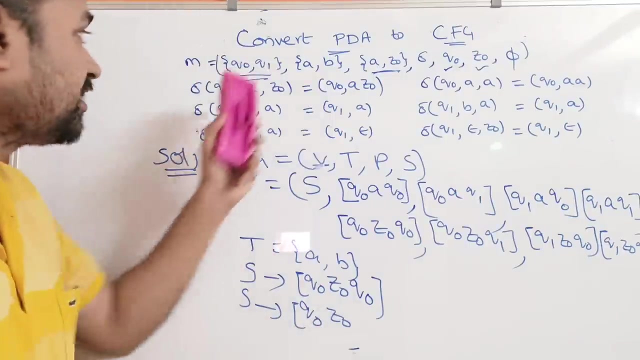 z naught. and what are the states? here we have two states, So first for this one we have to write q naught. So next one s implies here the initial state is q naught and initial symbol in the stack is z naught. So q naught, z naught. and what is the next state we have? 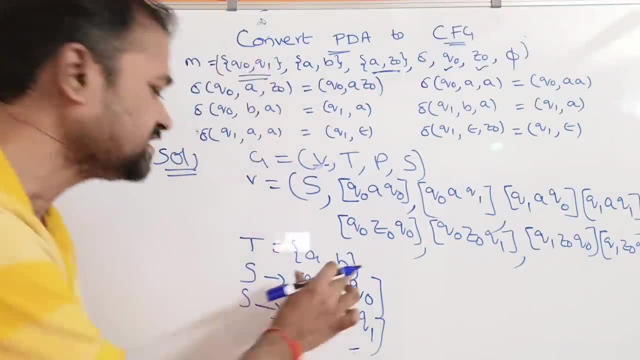 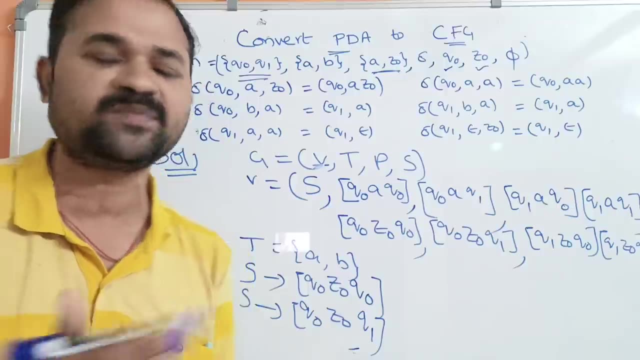 q 1, q 1.. So this is nothing but start symbol, start symbol productions. So till now we have written So context free grammar means we have to use four tables, So variables. so variables are written next to terminals, terminals are written next to start symbol. 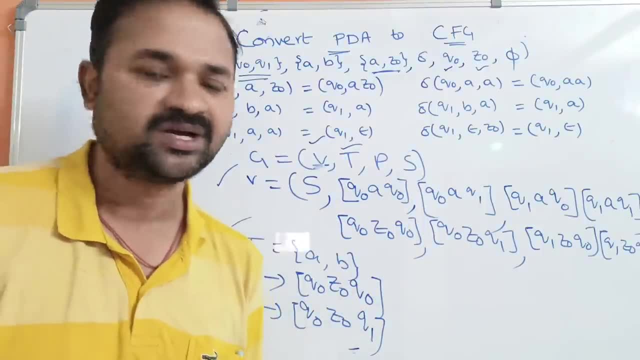 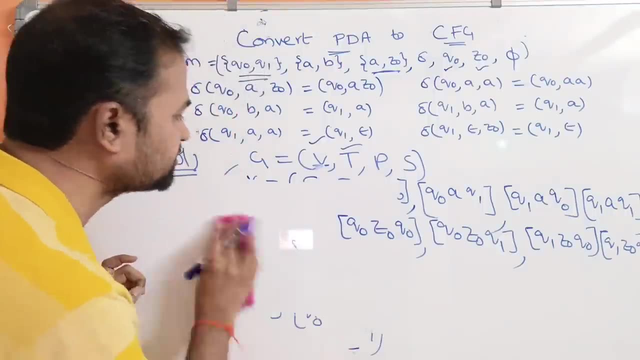 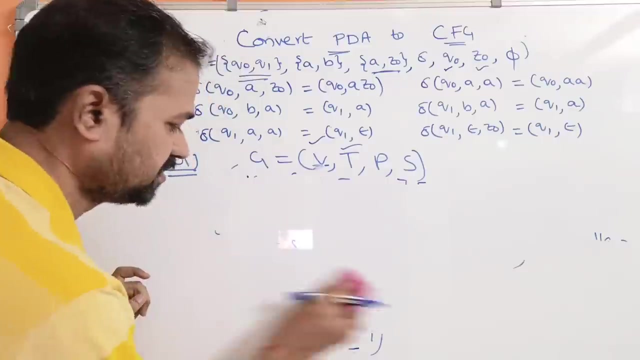 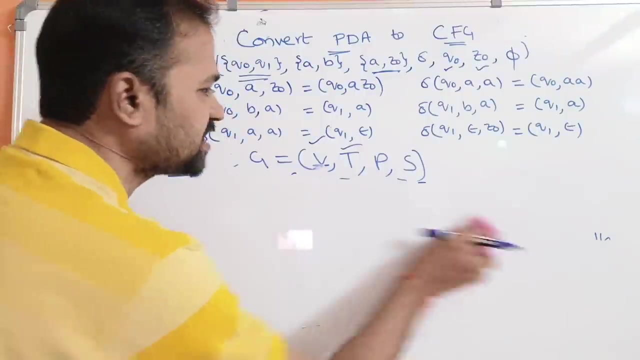 start symbol is written. Now we have to write the productions. So let us write the productions now. So for space constraints, I am erasing this portion. So let us erase variables, terminals, variables. So we have to write the productions. So, totally, 1, 2, 3, 6, 6, transition functions are: 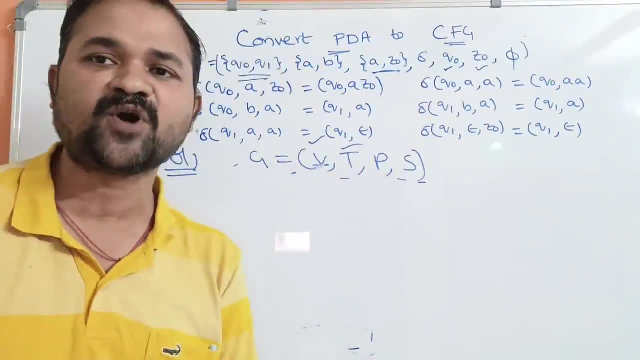 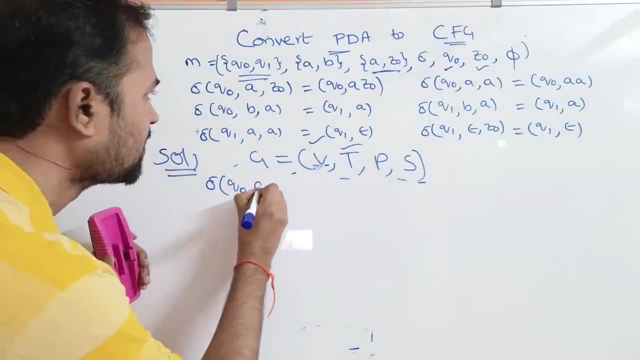 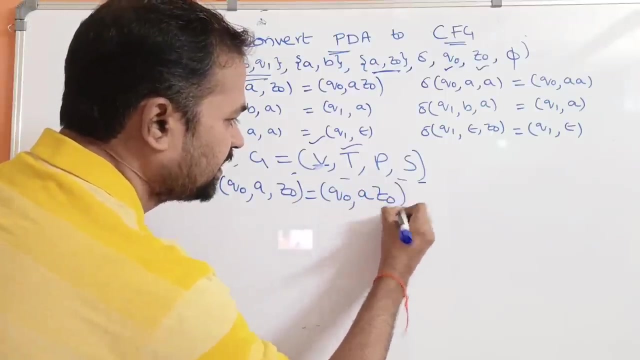 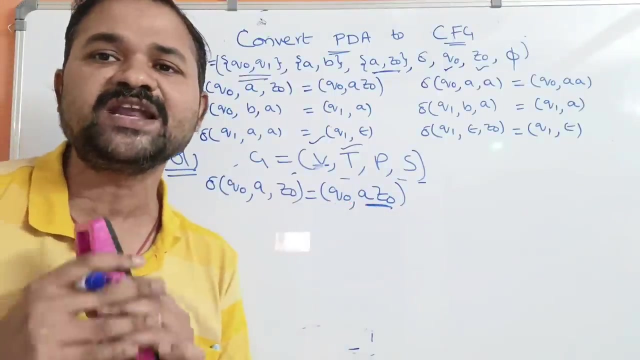 given. So for all those functions we have to write the corresponding productions. Let us consider the first two productions. delta of q naught comma a comma z naught is equal to q naught comma a z naught. Next, let us write the players. So let us write two with data equals 1, 1, 2, 3, so 3, which. 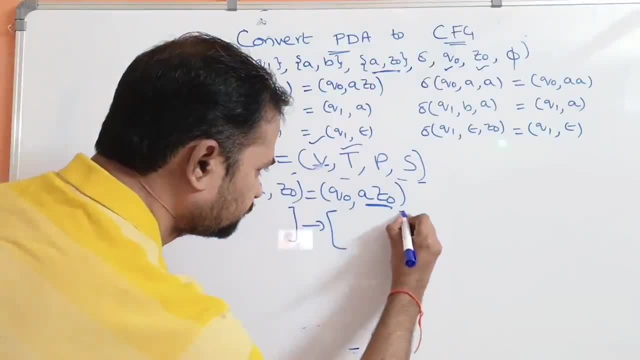 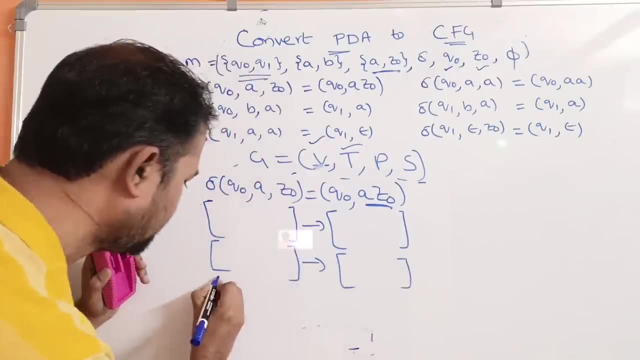 is equal to 5.. Next, we have also written the 4th part of theseHO如果 we refused to leave the stack, we can write that the stack totally contains two symbols. if there two symbols in the stack, then totally we have to write four productions. So this is the first two production. 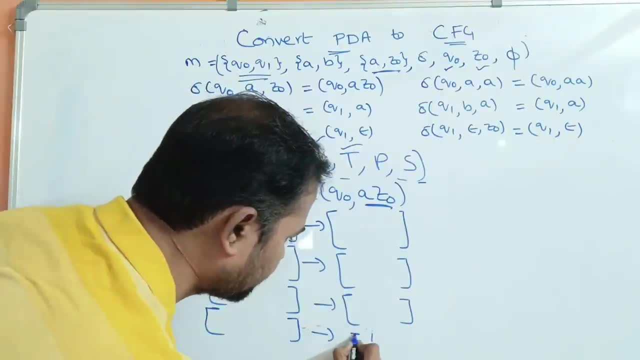 first two production. Next, 2nd production, second production, next, third one, 3rd one, next, let us write the 4th one. let us write the fourth one, 3rd one, 4th, So this is fourth production. Why? Because here the stack totally contains how many symbols. 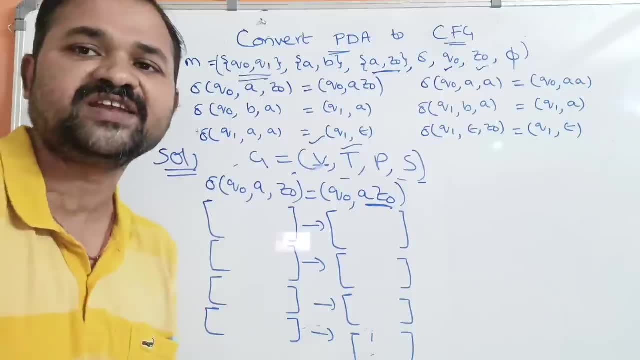 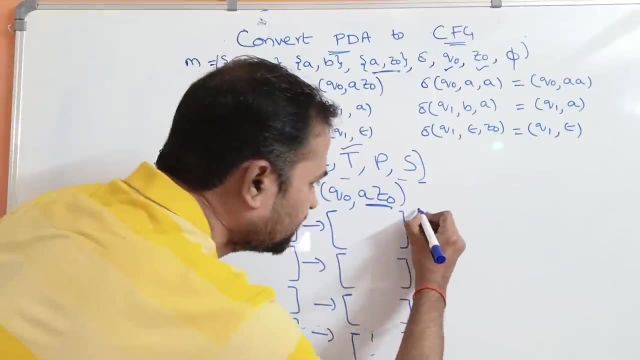 Four symbols. The stack totally contains two symbols, So that's why we need to write four productions Here. the stack contains two symbols, So that's why here at the right-hand side, we have to write two productions like this: 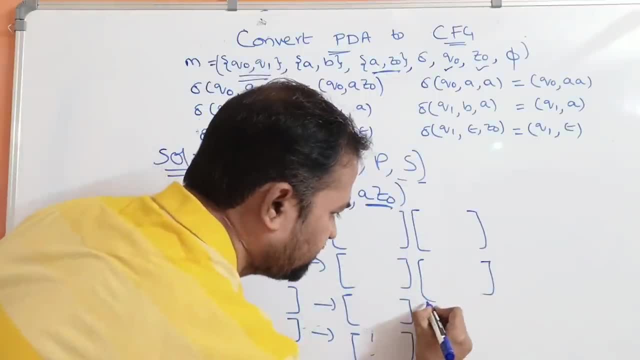 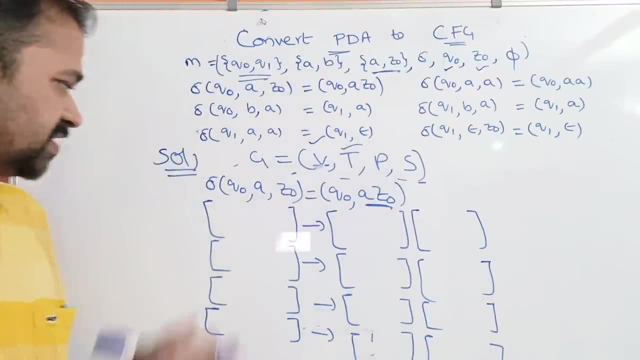 Why? Because stack contains two symbols. So that's why we need to write one more production here in the right-hand side. So next let us fill this one. So here the state is Q0.. So we have to write Q0 here. 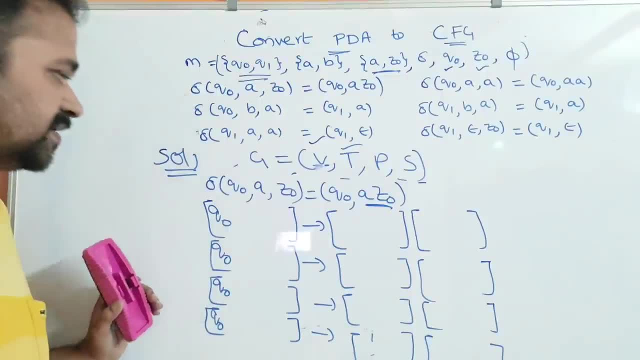 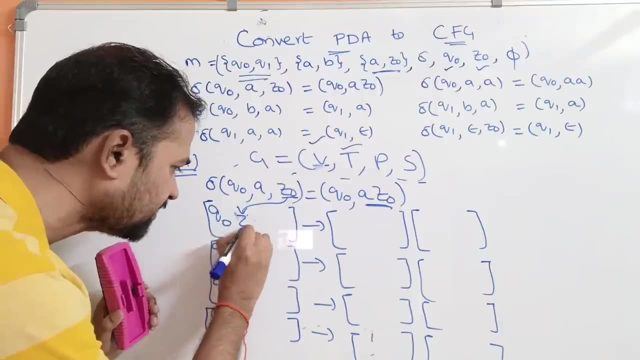 So in all the productions we have to write Q0.. Next, here the stack contains Z0. So this Z0 will be written in the middle. This Z0 will be written in the middle. So Z0,, Z0, Z0, Z0, Z0. 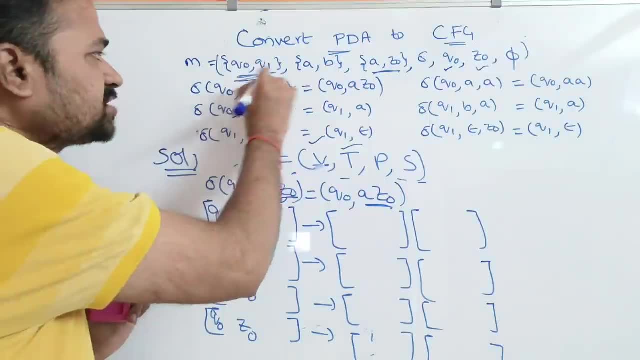 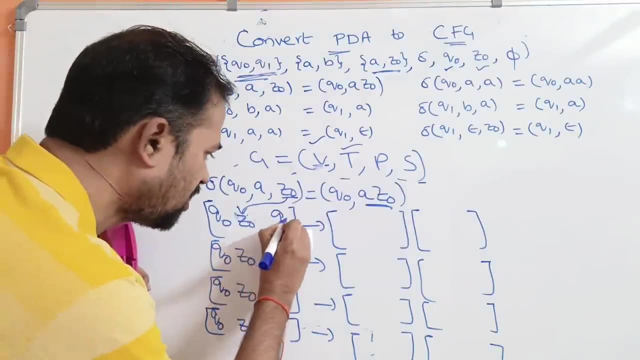 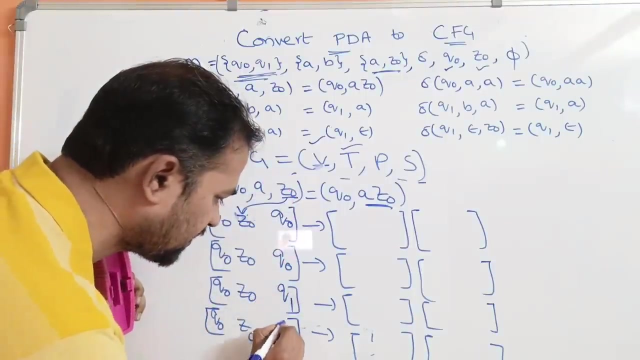 So next, here we have two states. What are those two states? Q0 and Q1.. So let us write those two states, So Q0, Q0.. So let us write Q0 twice, Next Q1, Q1.. 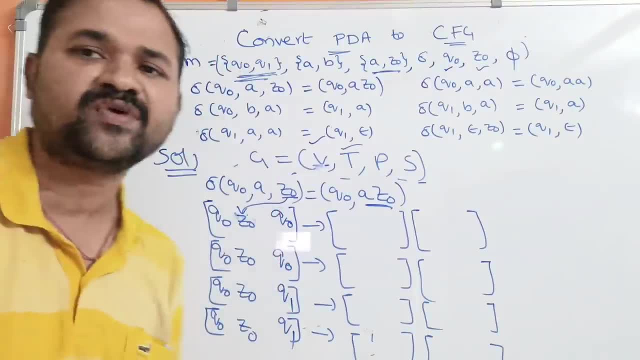 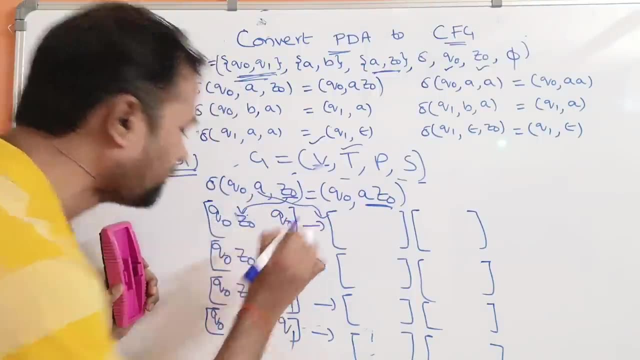 So let us write Q0 twice, After that write Q1 twice. Okay, Next one. Here we have A as the terminal symbol, A as the terminal symbol, A as the terminal symbol. Let us write. Let us write. 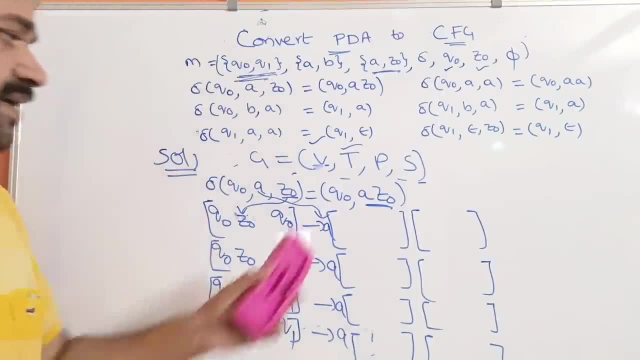 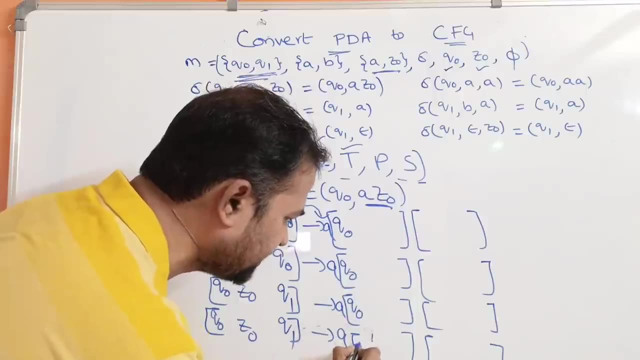 Let us write this A here. Let us write this A here. Next, here we have Q0 state. So let us write Q0 here. In all the productions, let us write Q0 here, Q0.. So next, here we have A Z0. 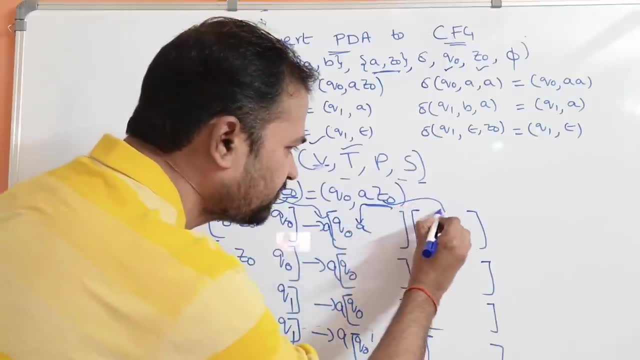 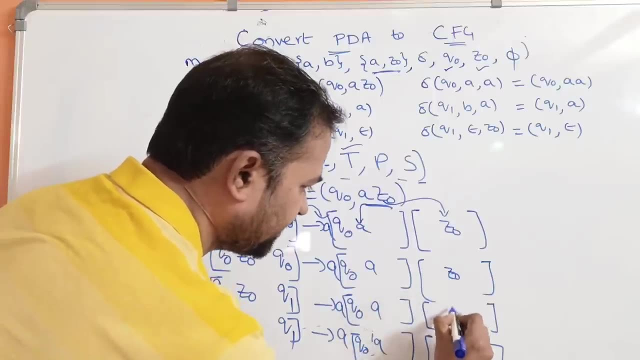 So this A will be written here in the middle. This Z0 will be written in this middle. Okay, So let us write A here. Next, let us write Z0 here. Let us write Z0 here, Okay, Next here: what are the states we have? 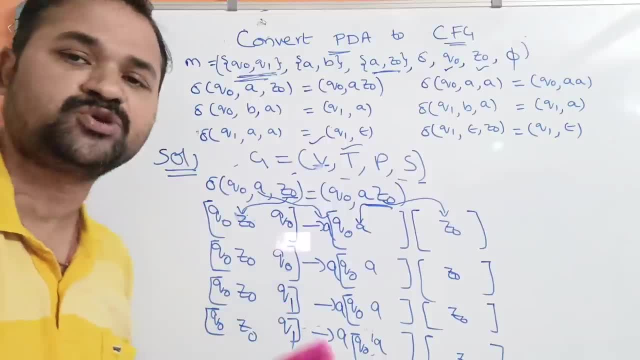 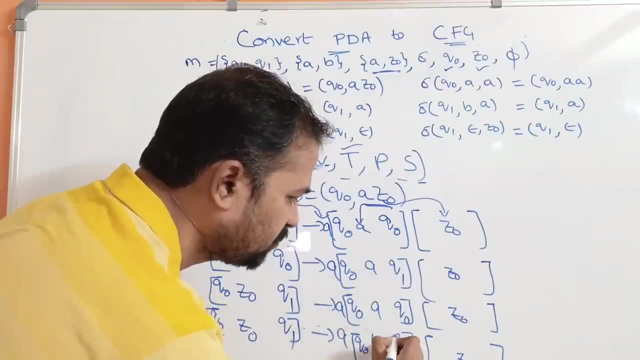 Q0, Q1.. Here we have written as Q0, Q0, Q1, Q1. Varias: here we have to write as Q0, Q1, Q0, Q1.. Here first we have written Q0 twice. 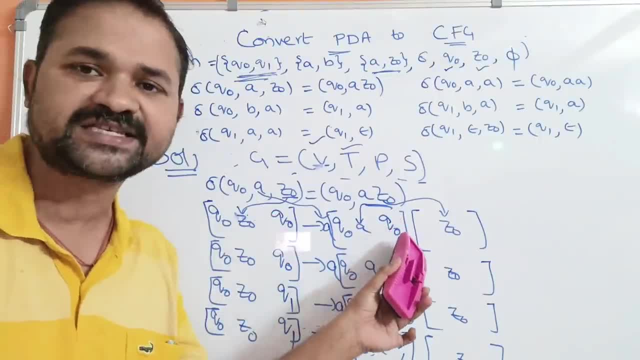 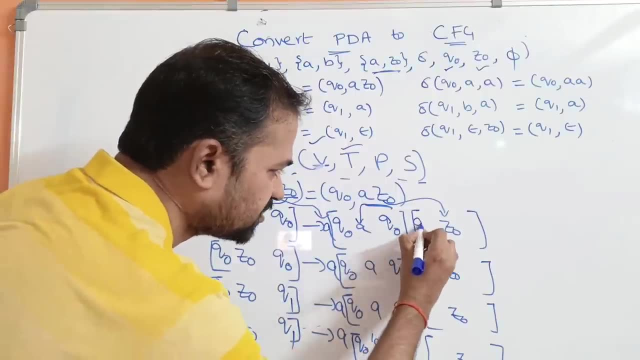 Next we have written Q1 twice Varias. here we have to write in this order: Q0, Q1, Q0, Q1.. Okay, Next here simply copy these productions here: Q0.. So copy this one here. 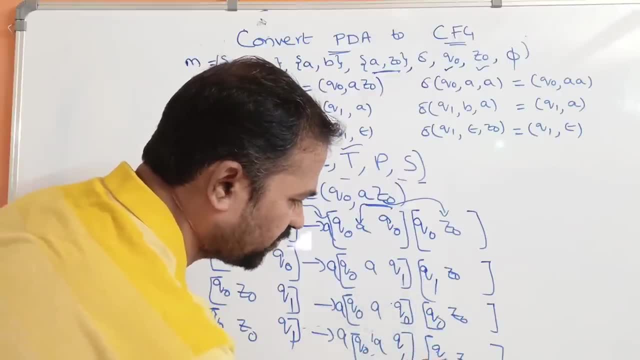 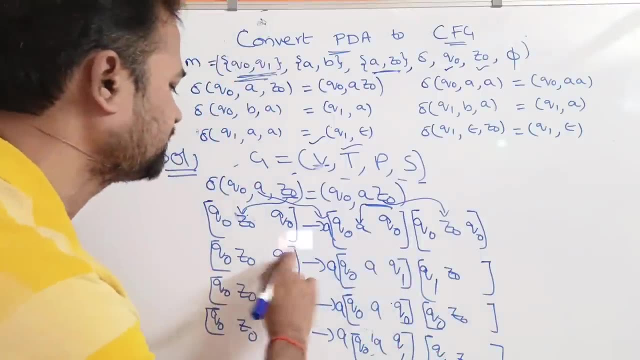 Q1.. So copy this one here: Q0.. Here, Q1.. Next here. simply, we have to copy these states here: So Q0.. So next one: Q0.. Next one: Q1.. So next one. 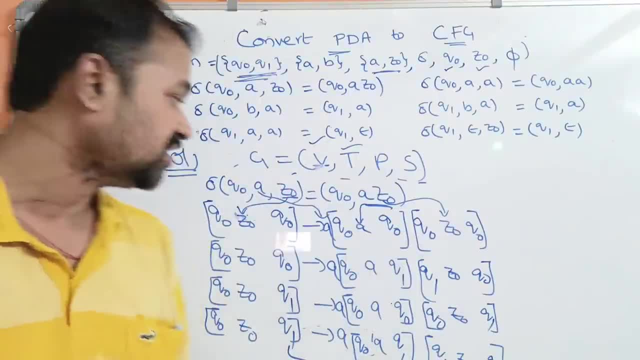 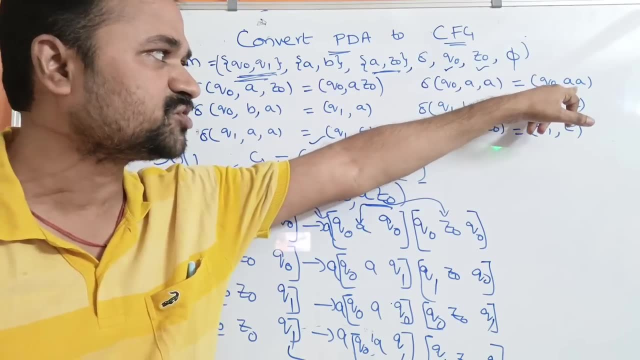 Q1.. So all these are the productions which are associated with this transition function. Okay, So now let us write for the next one. So here also, the stack contains two symbols. So this is: This is similar to this one only. 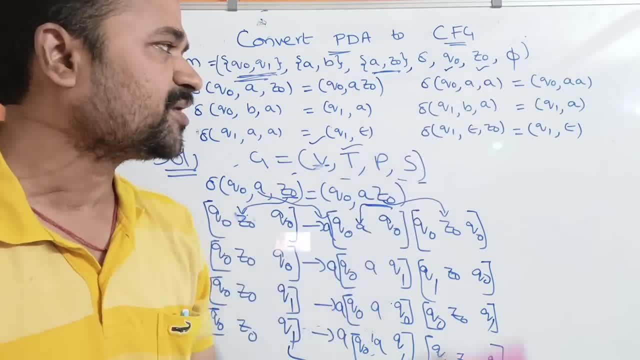 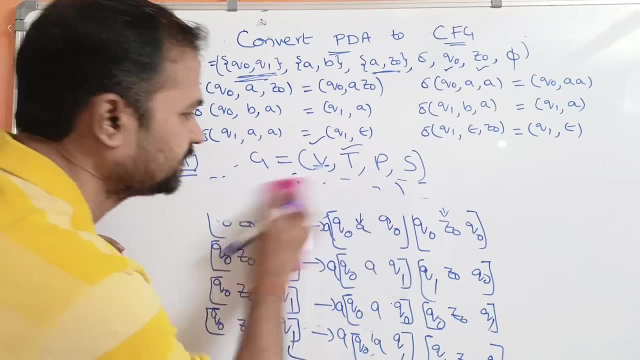 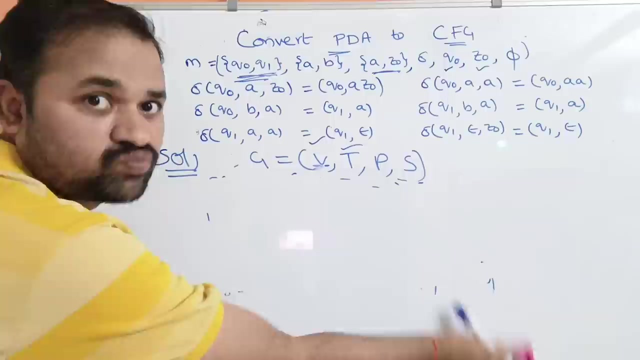 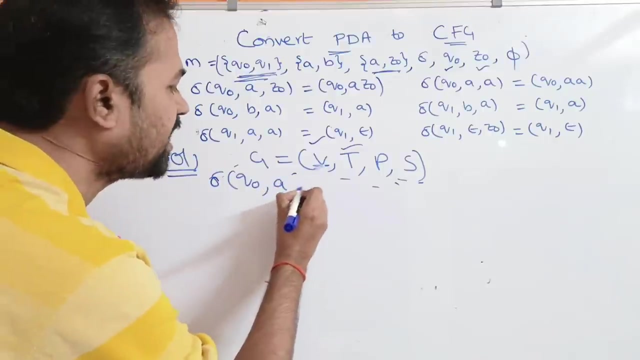 So if you have any doubts, then by writing the productions for this transition function, all those doubts will be clarified. Okay, All those doubts will be clarified. So what is the next transition function? Delta of Delta of Q0, A. A is equal to Q0, A is equal to Q0, A is equal to Q0. 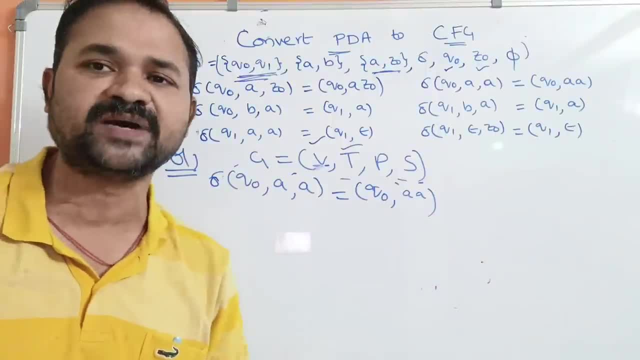 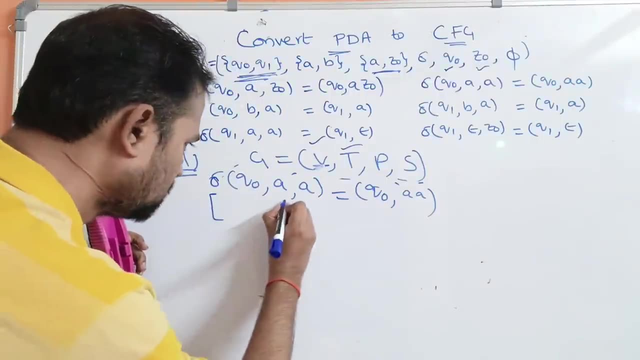 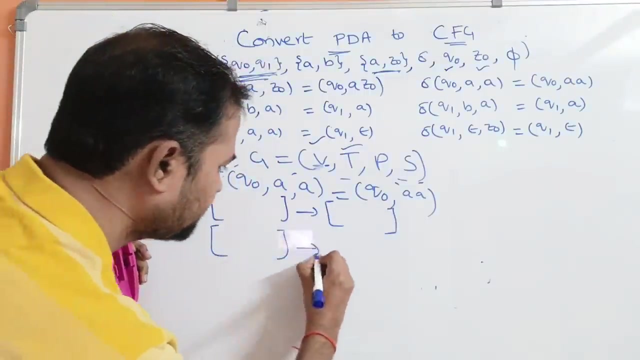 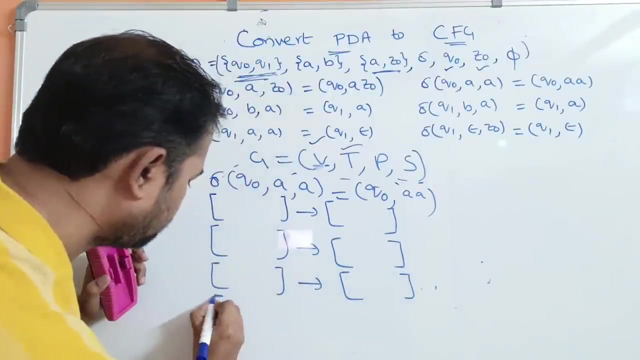 Okay, So here also, the stack contains two symbols. So if there are two symbols, then totally we will get four productions, Four productions. So this is the first production, Next is second production, Next third one, Next fourth one. 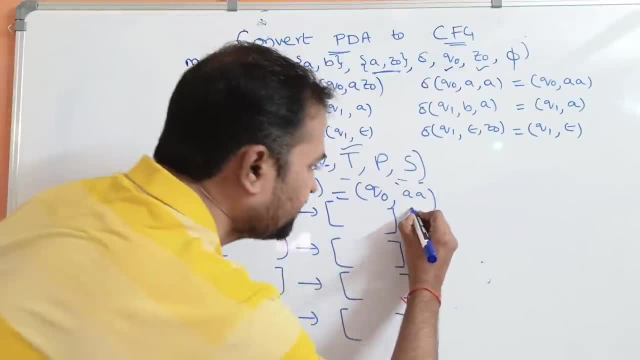 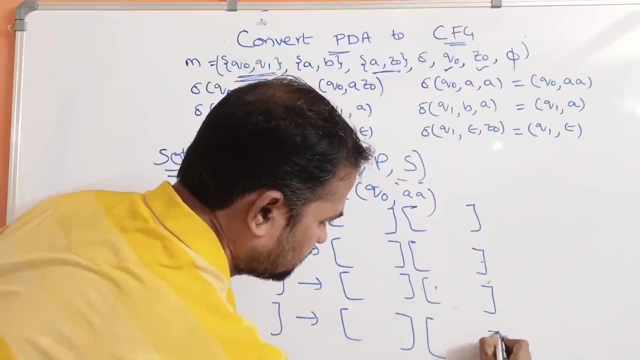 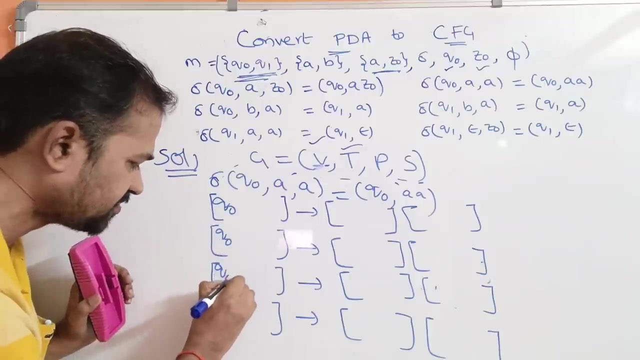 Here the stack contains two symbols, So that's why here we have to write one more production. Okay, So first year here we have Q0. So let us copy Q0 in all the productions Next year. the stack contains A. 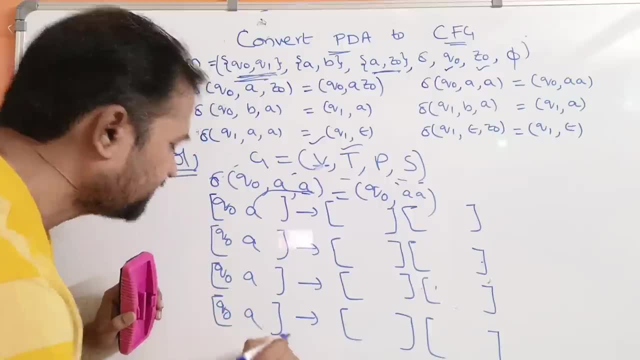 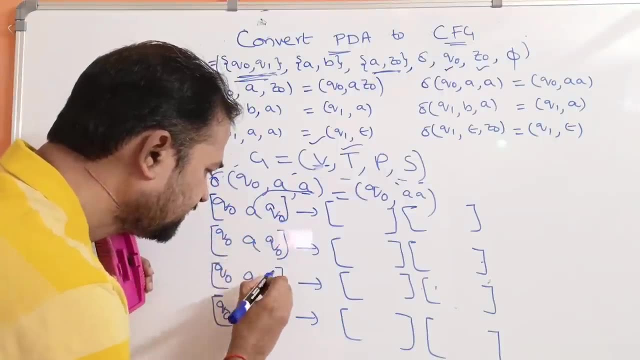 So let us write this A here, This A here Next year. we have two states, are there Q0 and Q1.. So let us write Q0.. Q0 twice, and then write Q1 twice Next year. here we have Q0. 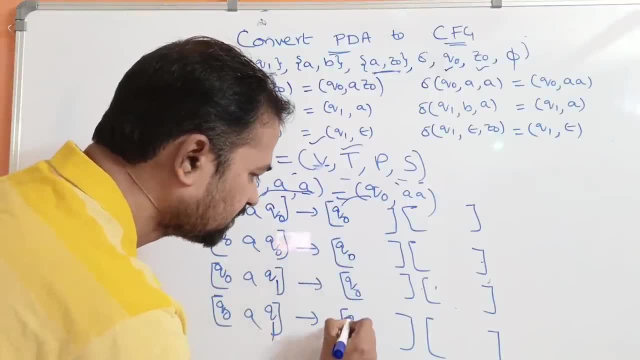 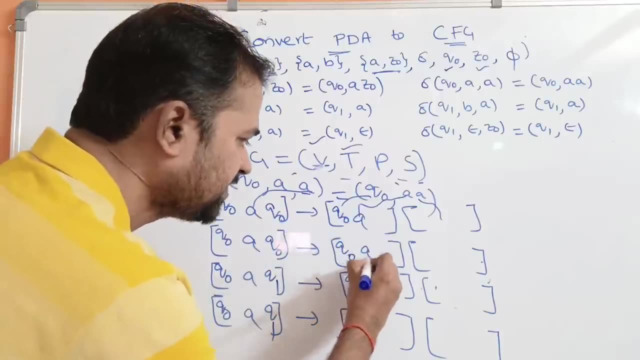 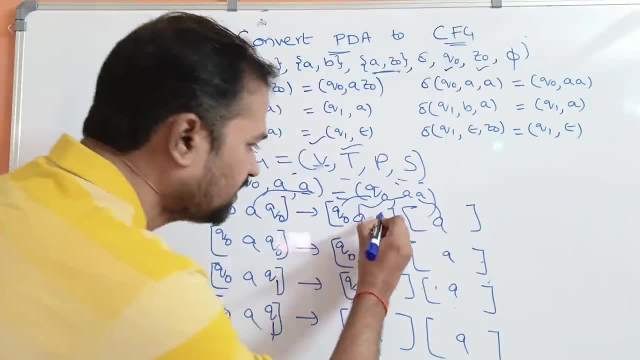 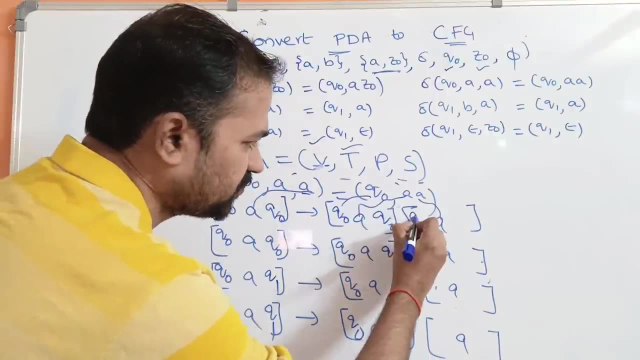 And here we have two states: Q0, Q1. So write here as Q0, Q1. Q0. Q1. So let us copy this one here also, So Q0, Q1.. Next one: Q0, Q1.. 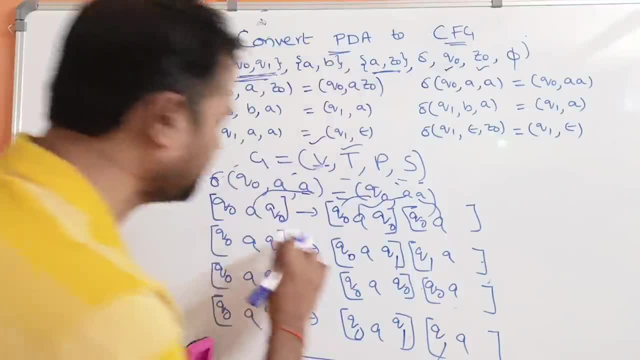 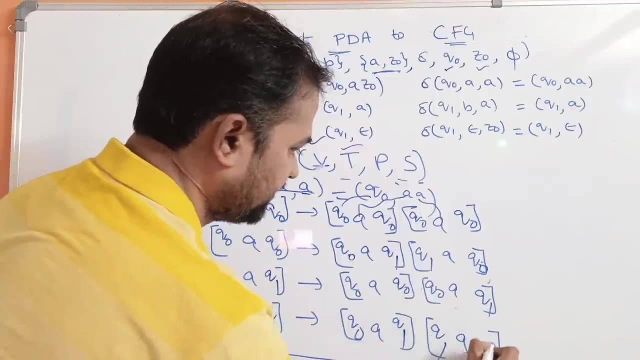 So next we need to copy all these productions here also all these states: So Q0, Q0.. Next to Q1.. Next to Q1.. Here we have A as the terminal symbol, So this A will be copied here. 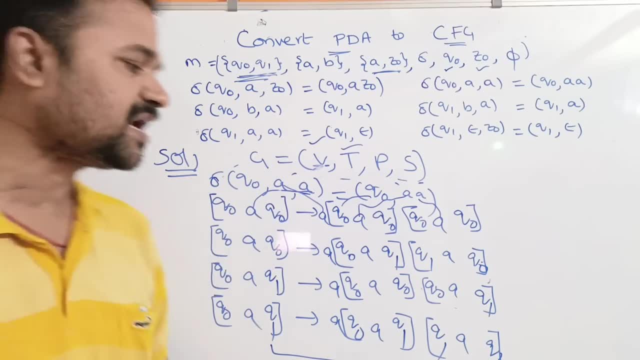 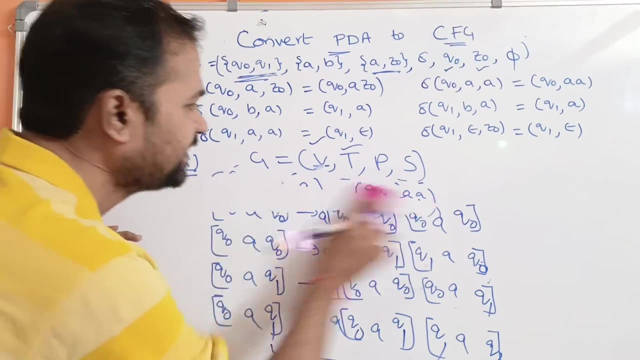 A, A, A, A. So these are the productions associated. So these are the productions associated with this transition function. So, likewise, let us write the productions for the next two transition function. So what is the next two transition function? 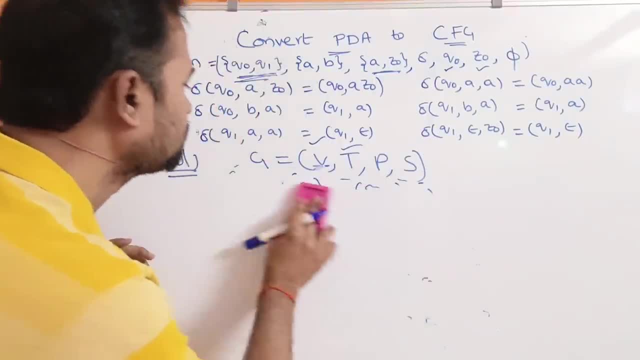 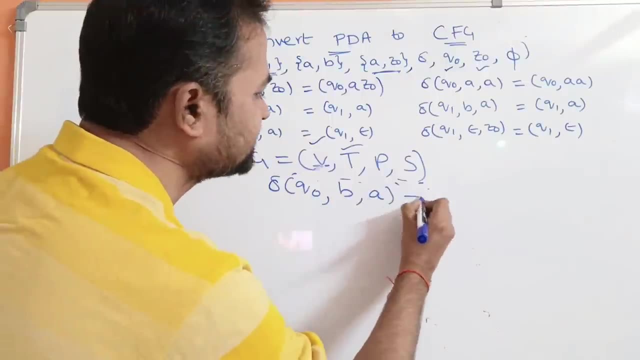 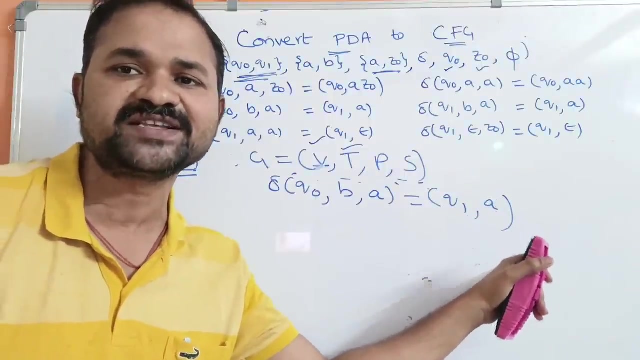 Q0, B A is equal to Q1, A. So delta of delta of Q0, B A is equal to Q1, A. Here the stack contains only one symbol. So if there is only one symbol, then we will get 2 power 1.. 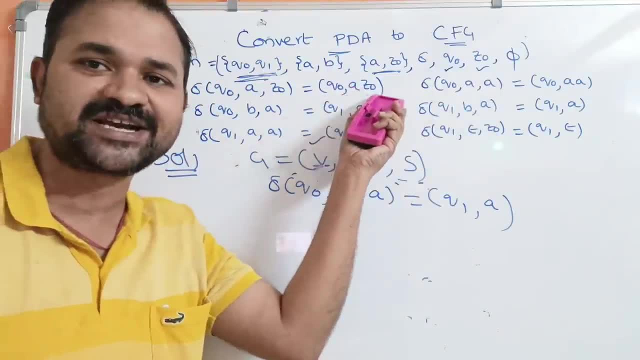 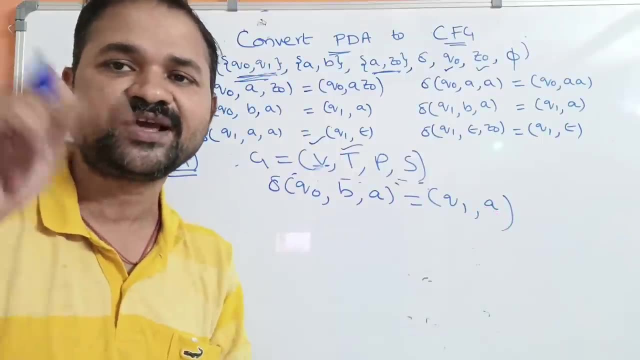 So two productions. Here the stack contains two symbols: C, A, Z, 0.. So that is why it contains 2 power 2, four productions. But here the stack contains only one symbol. So we will get 2 power 1, two productions. 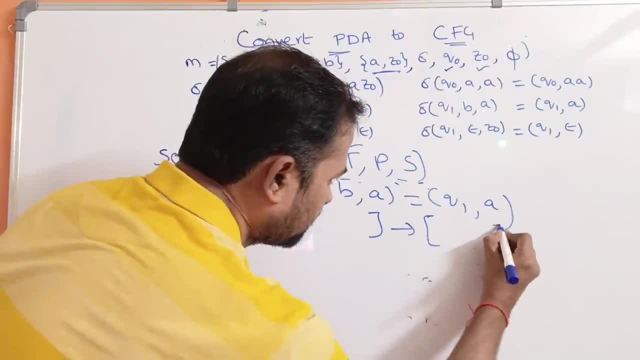 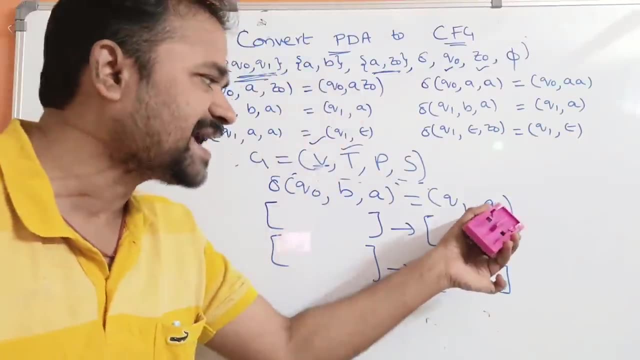 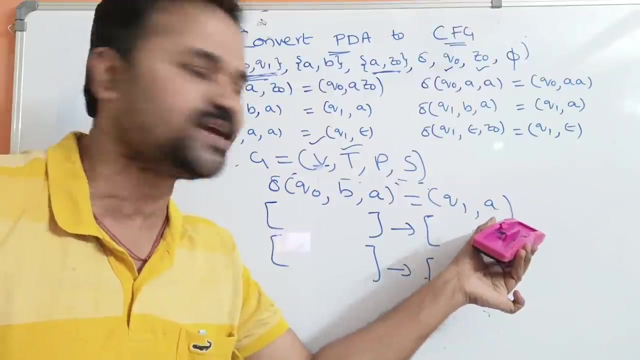 So this is the first production And this is the second production. This is the second production Here. the stack contains only one symbol, So this is enough. There is no need to write one more square bracket here. Why? Because the stack contains only one symbol. 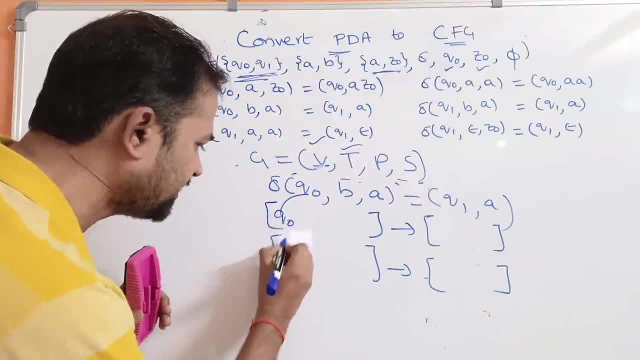 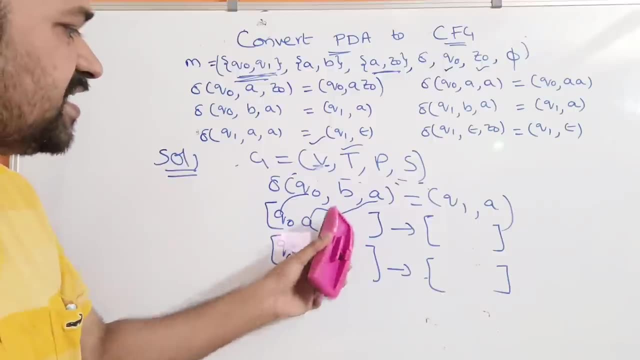 Okay, So let us write now So Q0.. Let us write Q0 here. Next year A. So this A is copied here. This is A. Next year. we have to write the states Here. we have two states, are there? 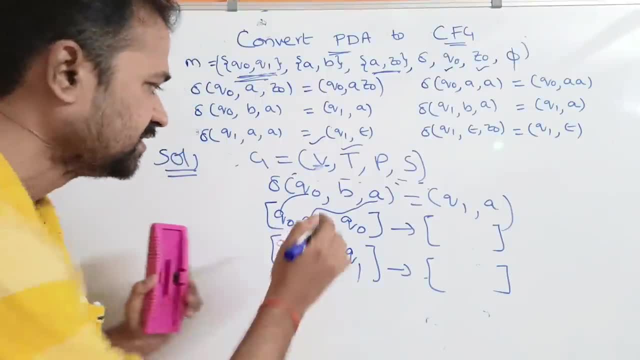 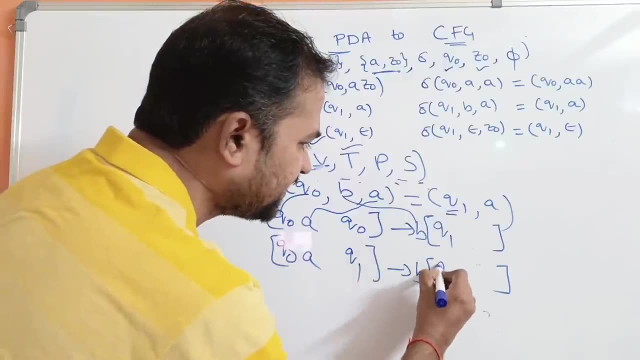 So Q0, Q1.. So let us write those two states. Next year the input symbol is B, So this B will be copied here. Next year the state is Q1.. So let us write that Q1 here. 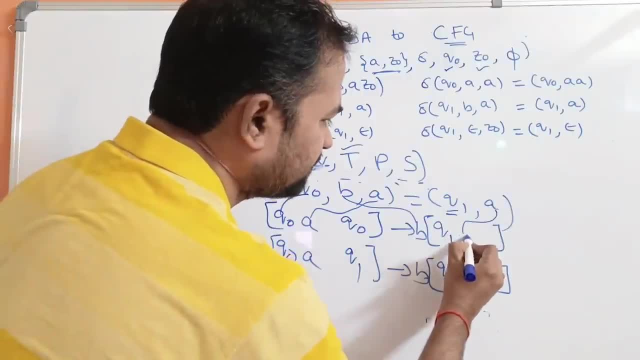 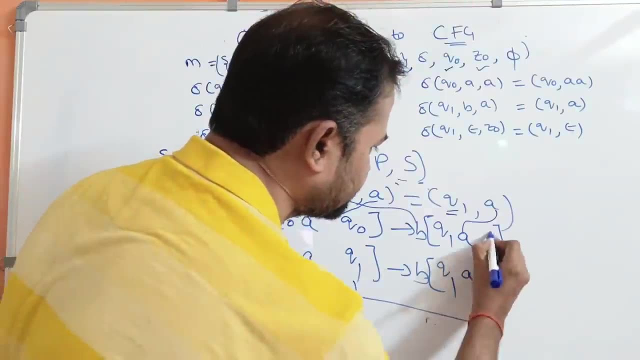 Next, Here we have only one gate, So let us write that A here, And next year let us write the states. So what are the states here? Simply, we need to copy the states. So Q0, Q1.. 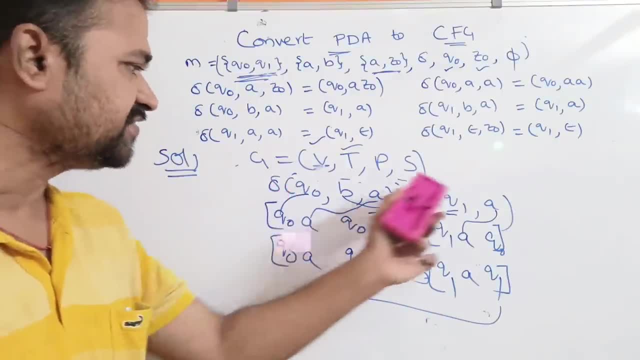 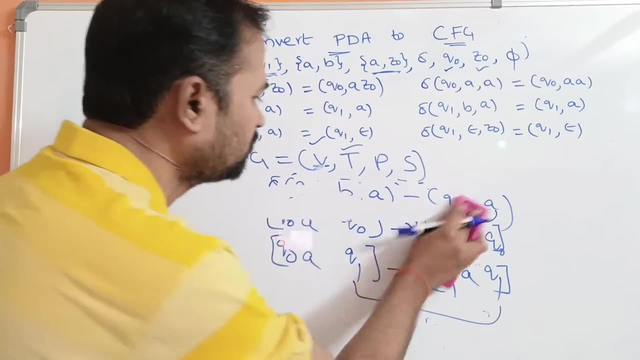 Q0, Q1.. So these are the productions associated with this transition function. So we can write the next transition function as this one. only So. fourth and third transition functions are same, only So. now let us write the transition function. 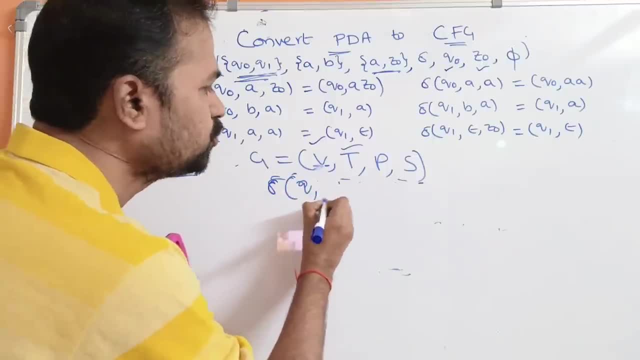 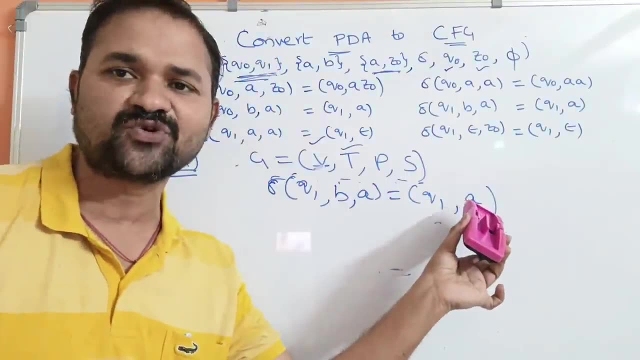 So what is the transition function? Delta of Q1, B, A is equal to Q1, A, So here also the stack contains only one symbol. So we will get 2 power 1. So two productions. 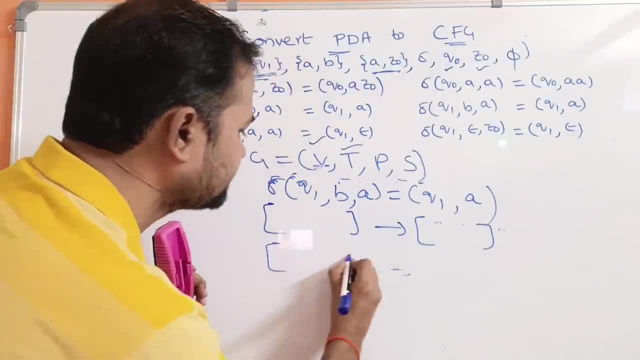 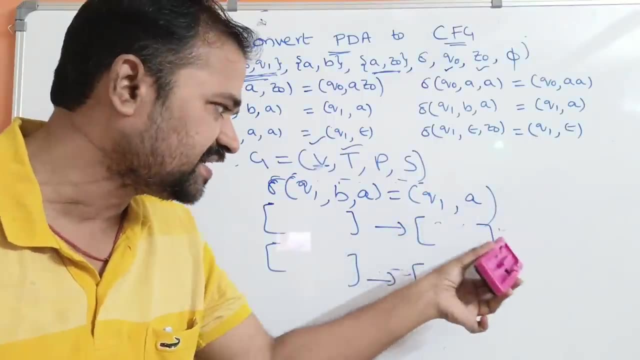 Two productions. So this is the first production And this is the second production. Okay, Here after comma, the stack contains only one symbol. So that is why here this only one square bracket is enough. There is no need to write one more. 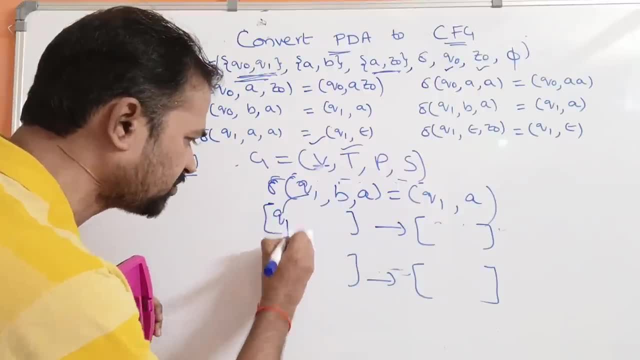 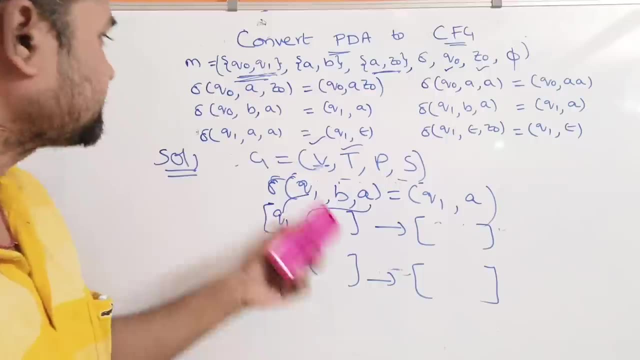 One more. So this is the first production, So let us copy this one here: Q1, Q1. Next. Next, here, the stack contains A. Let us write A here. Next, here we have two states. are there? 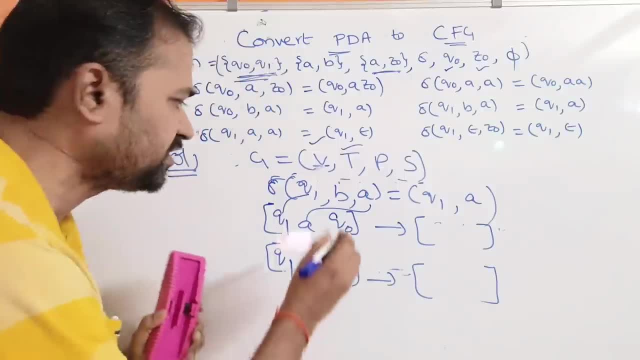 Q0, Q1.. So let us write those two states: Q0, Q1.. Here the terminal symbol is B, So let us write B here. Next, here the state is Q1.. Let us write Q1 here. 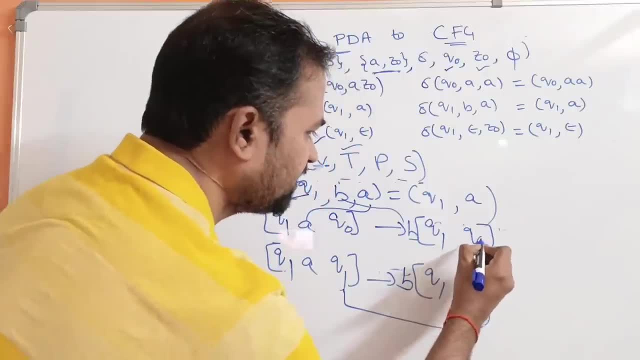 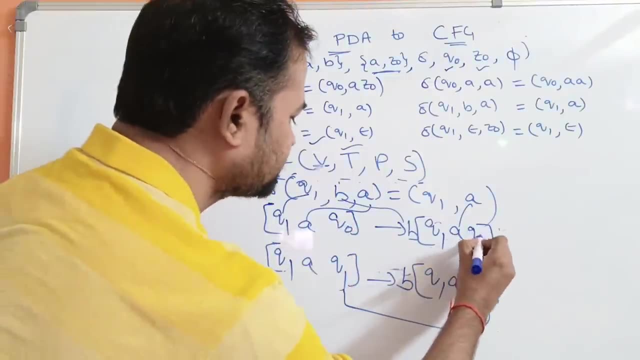 And next simply copy these states here, Simply copy. I am sorry, Here we need to write A, A, A A. Next, simply, we need to copy the states: So Q0, Q1.. So Q0, Q1.. 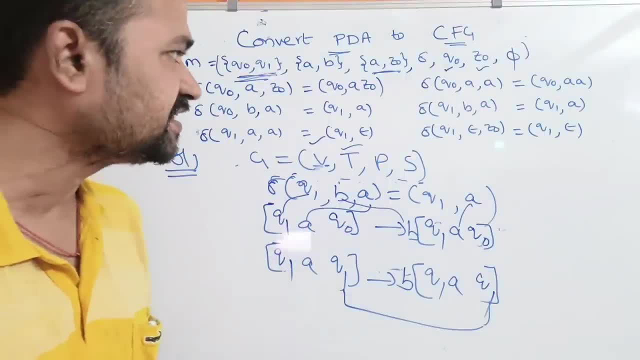 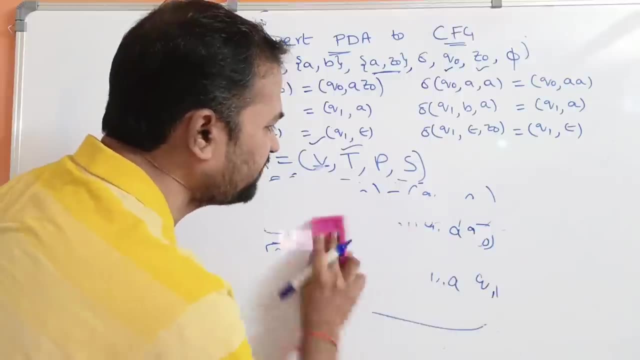 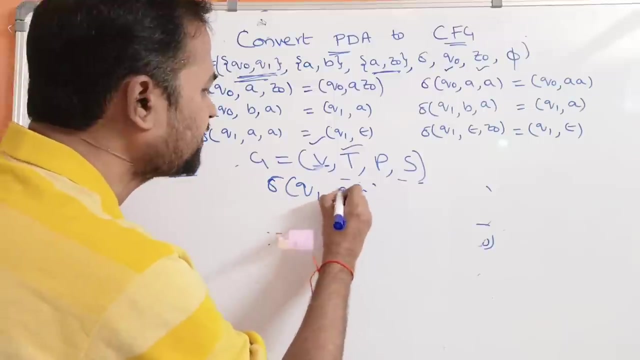 So these are the projections associated with this transition function. So now let us write the projections for the remaining two transition functions also. Delta of Delta of Q1 comma A. comma A is equal to Q1 comma epsilon- Q1 comma- epsilon. 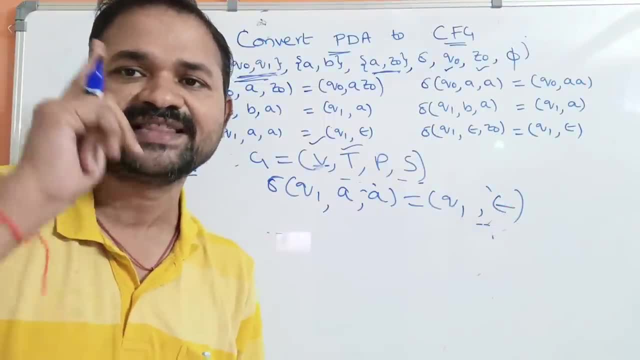 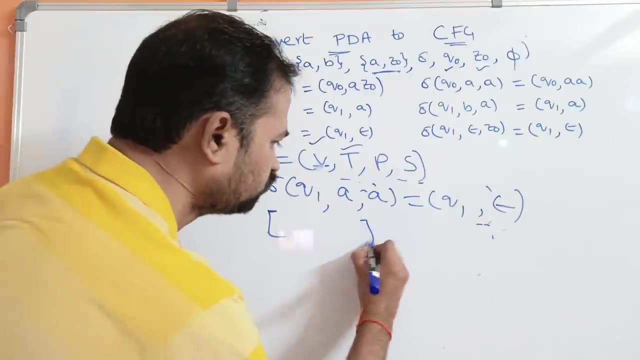 Here the stack contains epsilon. If we have epsilon, then we will get only one production. If we have epsilon, then we will get only one production. Okay, So this is that production. So here we have epsilon. So only one square bracket is enough. 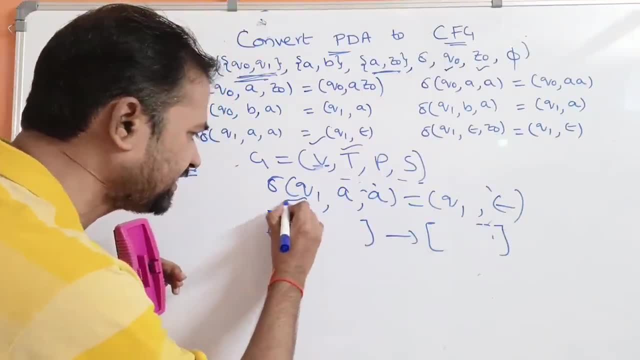 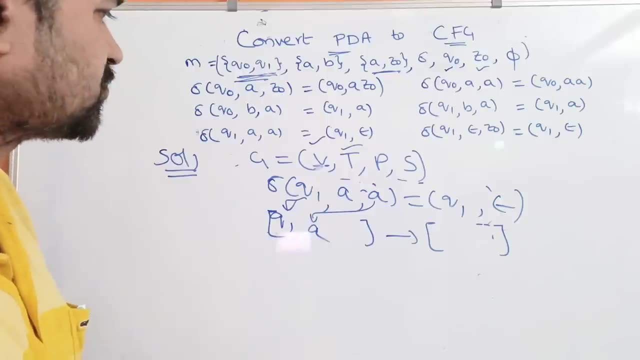 There is no need to write one more square bracket, So Q1.. Let us write: Copy this one Next. let us copy this one here. Next, here we have the states. So what are the states here Here? 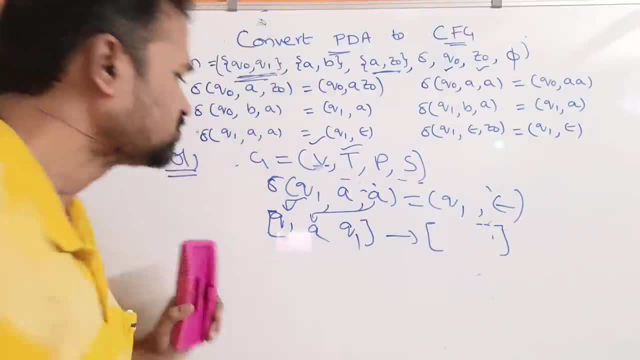 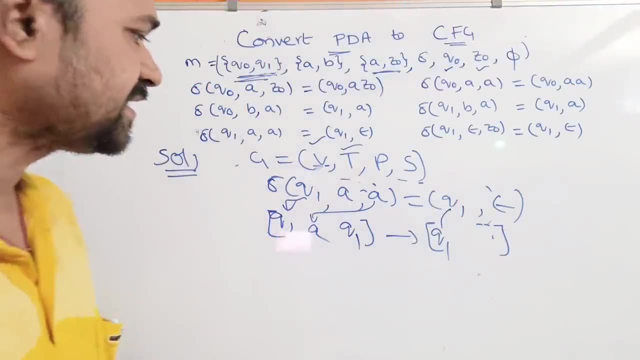 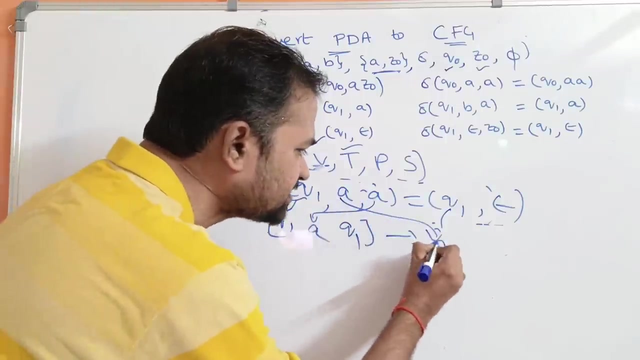 Here we have Q1.. So let us copy that state here. So Q1, A, Q1.. And let us write this Q1 state Next here here: here, if we have epsilon, then we have to write this terminal symbol here: 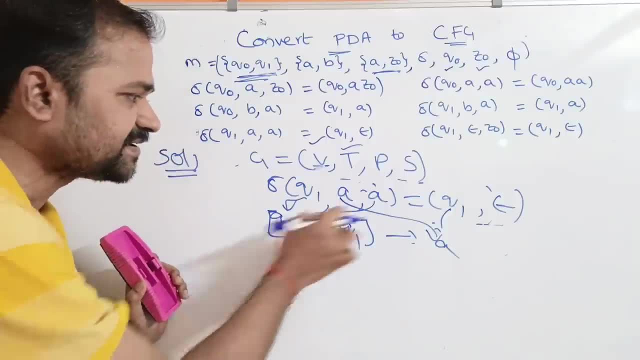 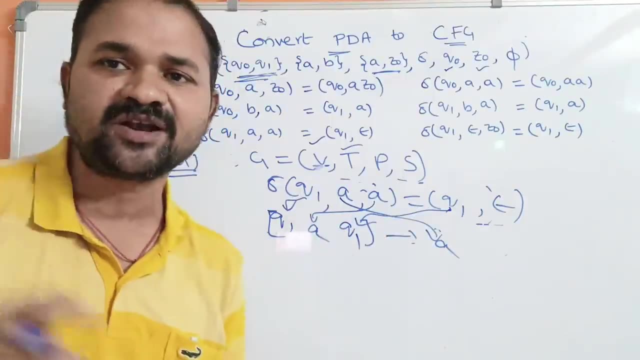 So let us observe one more time. So this Q1 is written here, Next this A is written here And this Q1, we have to write this Q1 here. If we have epsilon, then we will get only one product. 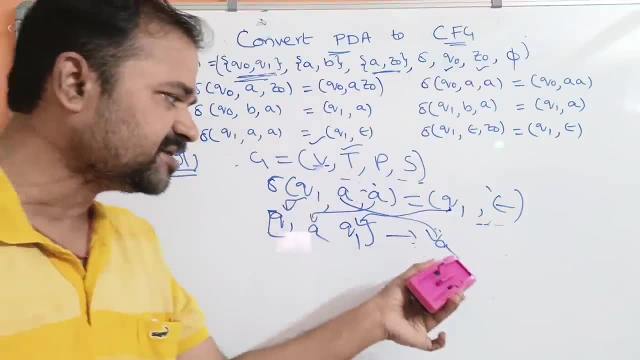 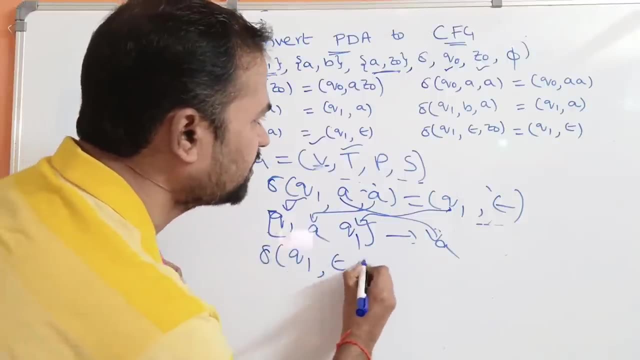 So let us copy this So we will get only terminal symbol. here In the middle we have terminal symbol. That terminal symbol should be written here. Okay, So let us write for the last one also: Q1, epsilon Z naught is equal to Q1, epsilon. 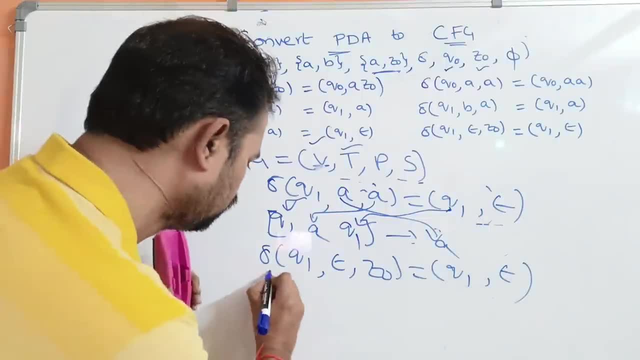 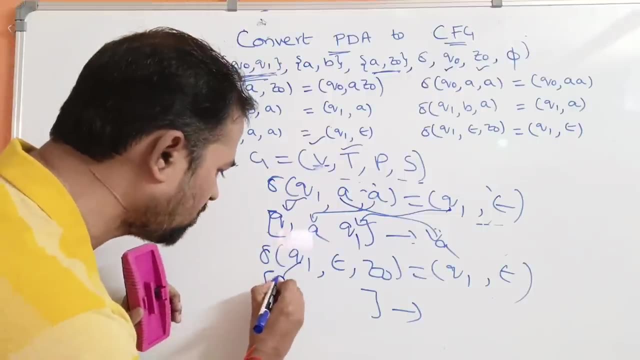 So here we have epsilon, So we will get only one production. We will get only one production Here. let us write that production. So let us copy this one here: Q1.. Let us copy this symbol here: Z naught.